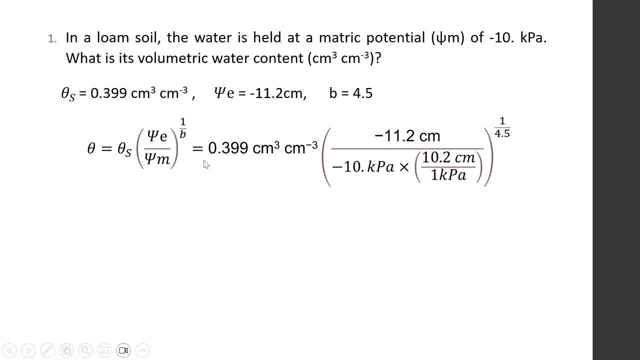 In getting the volumetric water content. we just need to plug in the values above. So a helpful conversion to remember when solving this problem is that 1 kPa is equal to 10.2 centimeters of water. So in this case we need first to divide the air entry potential, which is minus 11.2 centimeters. 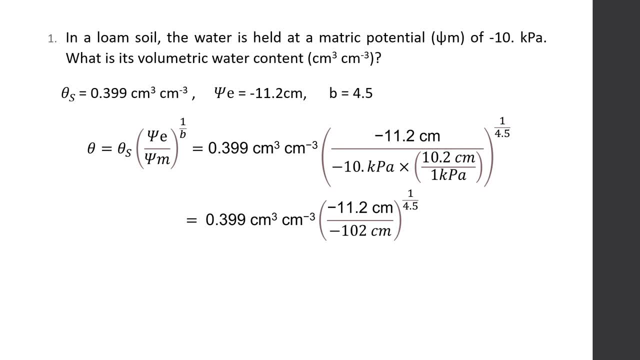 over the depth of water at minus 10 kPa, which is 102, minus 102 centimeters of water, And raise the quotient to 1 over 4.5, or 0.22.. Lastly, we will multiply the answer with the saturated water content, which is 0.399 cubic centimeter per cubic centimeter. 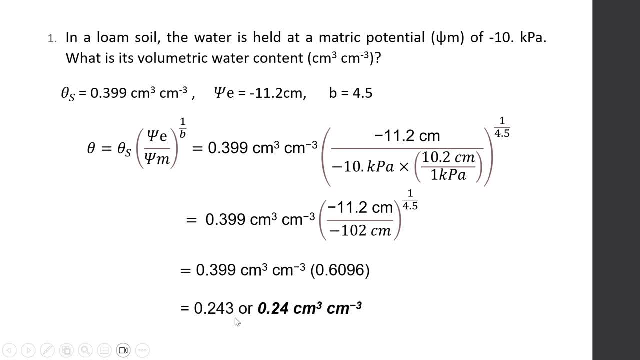 And we will arrive with 0.243 cubic centimeter per cubic centimeter, And we will arrive with 0.243 cubic centimeter per cubic centimeter, And we will arrive with 0.243 cubic centimeter per cubic centimeter. 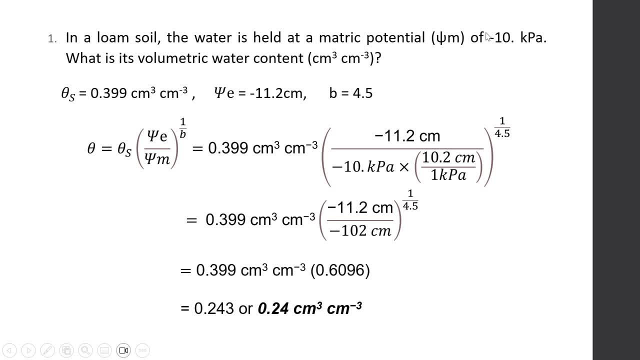 Take note that in the problem we're using 2 sig figs. therefore the answer should be reduced into 2 sig figs. So we have the volumetric water content of this loam soil at a metric potential of minus 10 kPa. 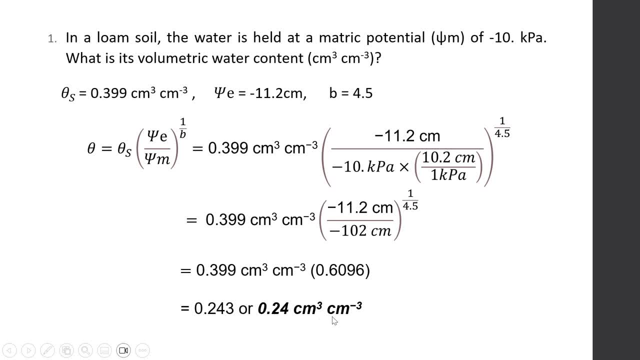 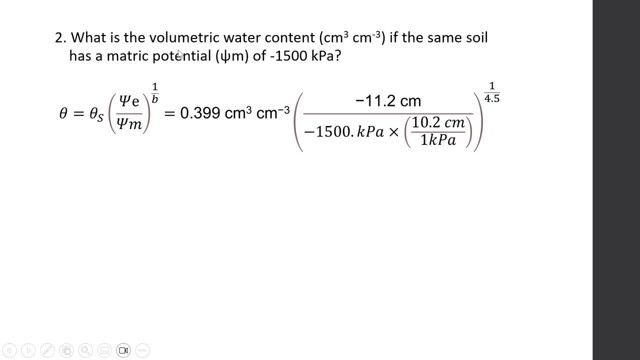 is 0.24 cubic centimeters per cubic centimeter. So number two: What is the volumetric water content if the same soil has a metric potential of minus 1500 kPa? So here the procedure is just the same with the previous problem. 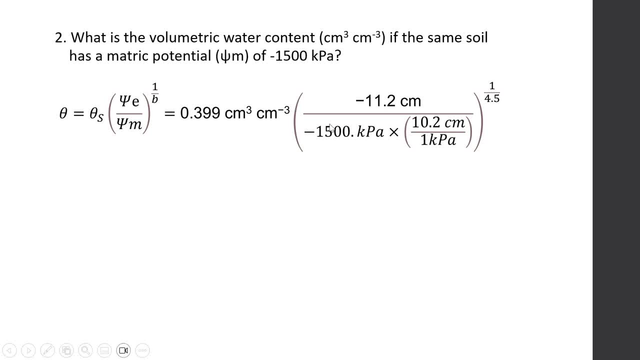 We just need to replace the metric potential of the soil from minus 10 kPa to minus 1500 kPa and do the same process. Just plug in the values and we will get the volumetric water content of the same soil at minus 1500 kPa.